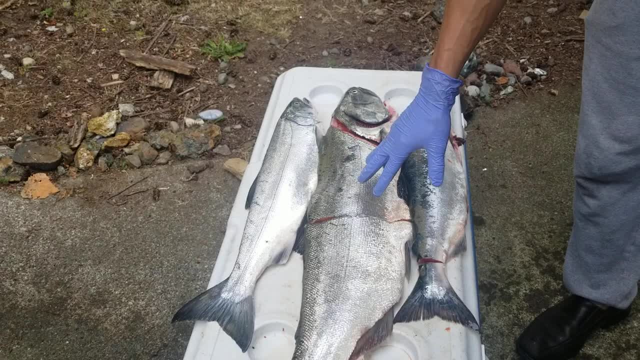 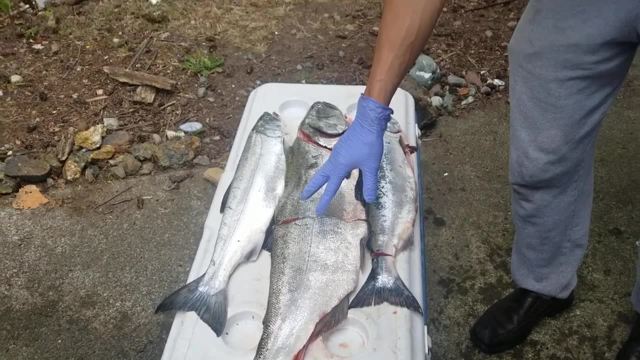 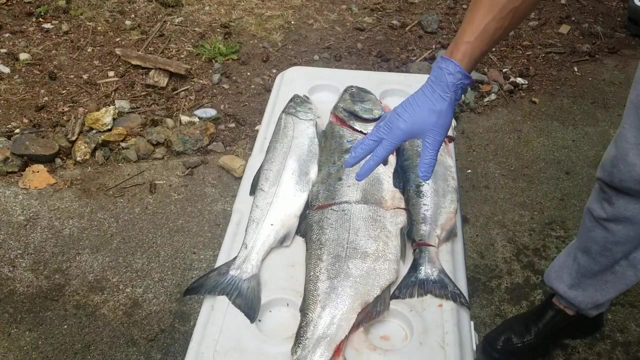 a fish this big- almost 100- it's going to be a king salmon. coho rarely get this big. pinks never get this big. i think the state record for pink salmon here in washington is something like 10 or 11 pounds. so another way to tell the difference, because oftentimes you might catch a wild coho. 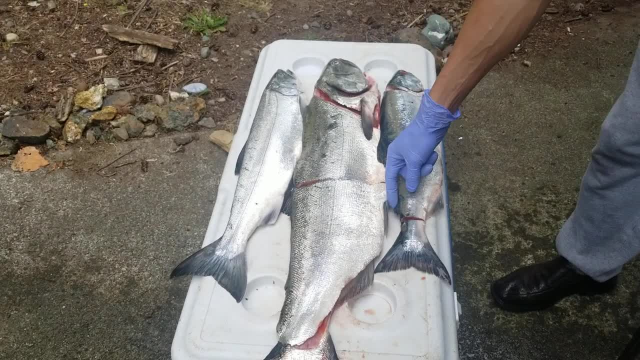 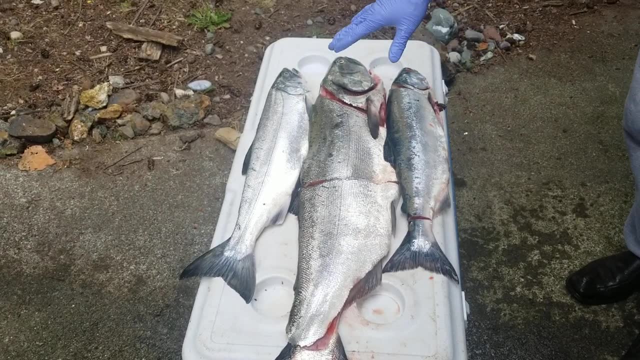 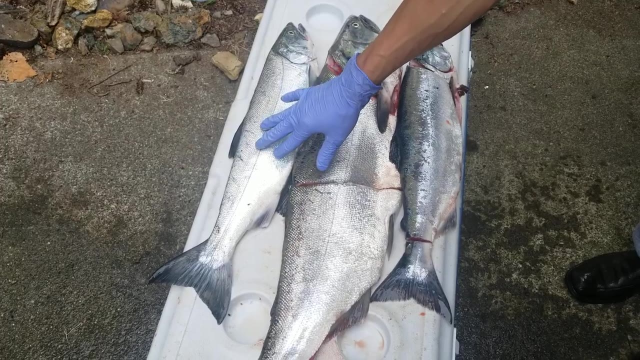 or silver salmon that has an adipose fin, like this pink salmon does right here. so how to tell the difference between these two fish? well, if you just look at the scales- that's typically what i'll look at- can you see how the scales here are really organized, and they're a little bit. 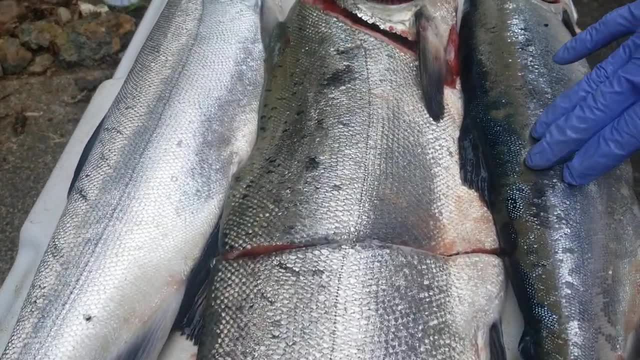 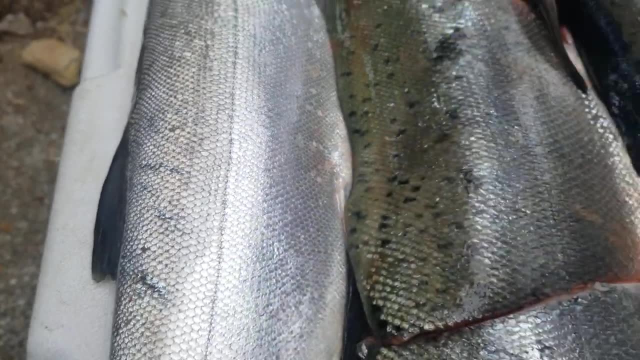 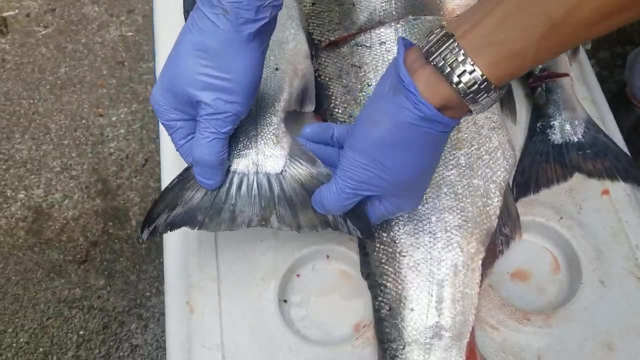 bigger than these tiny little pink scales on here, and the lateral line is more defined here on a silver salmon than it is on a pink salmon. another way to tell the difference is you look at the tail. can you see this tail here? and how there's this iridescent silver in it? 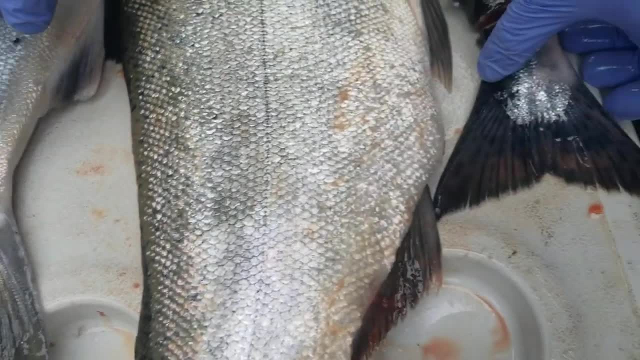 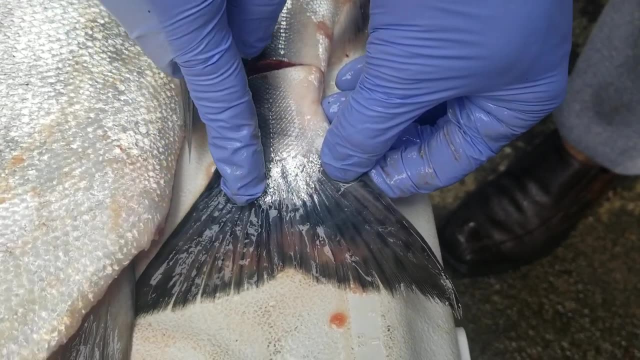 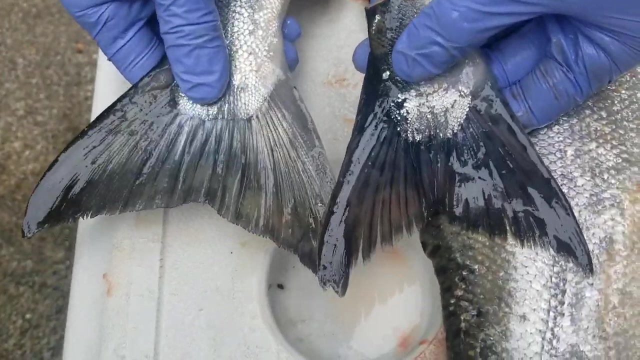 that's a way to definitely tell that you have a silver salmon. here is the pink tail right here and there's no iridescent silver in the tail. we cut the tail off here to be able to show you the two side by side. can you see the iridescent here in the tail, whereas you don't have that in the pink tail? 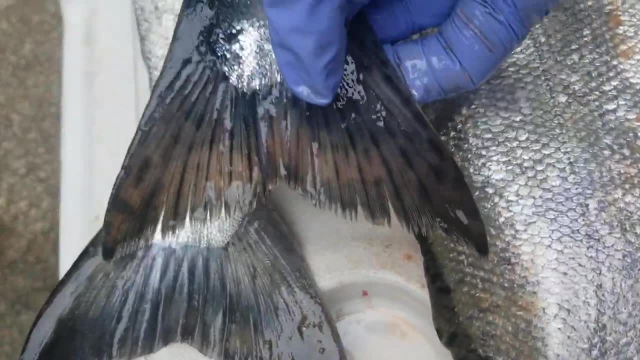 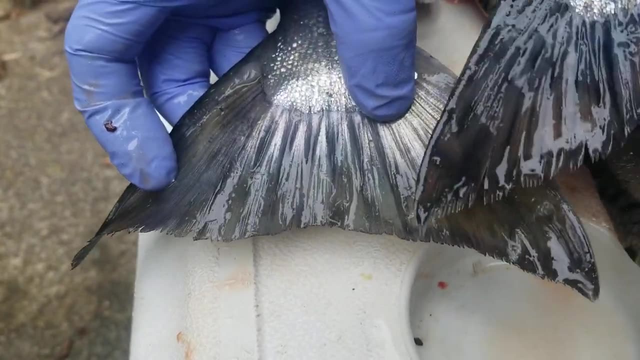 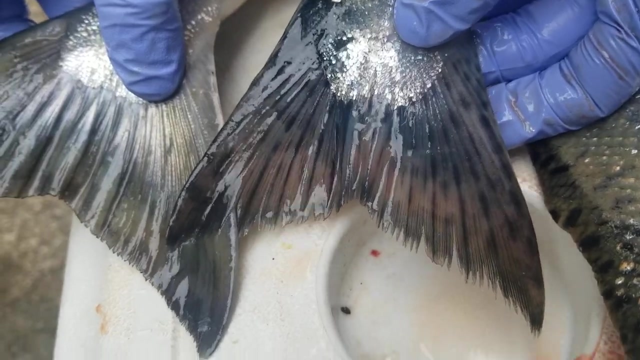 the pink tail has a bunch of big spots on it. if you can see that with the camera angle you don't have those spots in a silver tail. see those spots. are they hard to see? maybe you could see them better there. okay, so you can look at the tail. another thing is, you can look 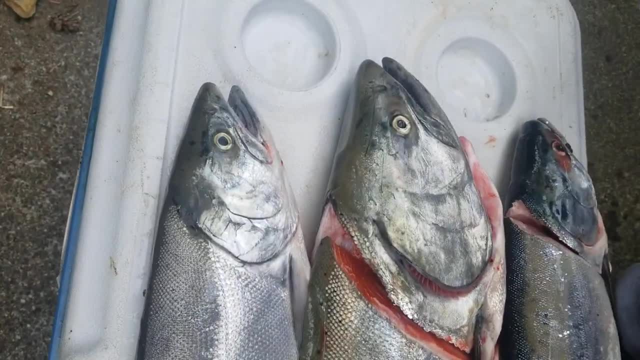 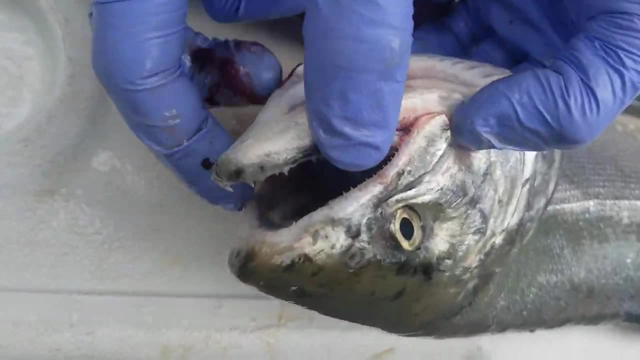 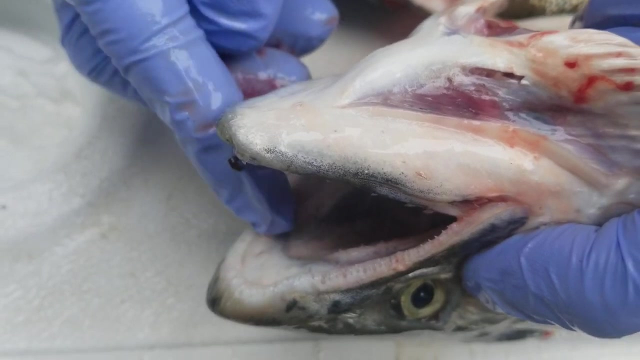 at the mouth. so if you come around to this side, you can see that the silver salmon have a bit of a white mouth and white gums. so you open it up and, yeah, a little bit white on the roof of the mouth- definitely white up here. we cut off the head of the pink and we'll show them side by side. 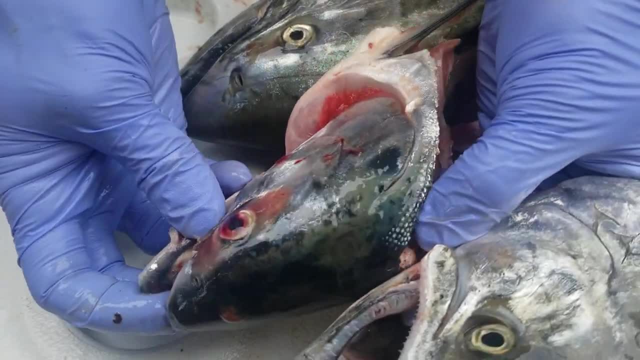 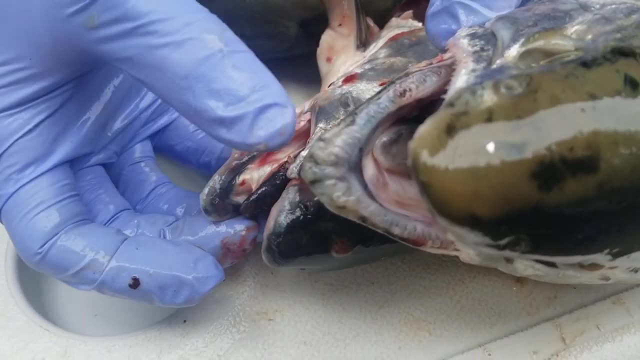 on the lower gums a little bit harder to tell, but you can see that the gums have a little bit of a white mouth and white gums on the bottom side. you can see how it's a little bit darker here on the pink than it is on this silver salmon.